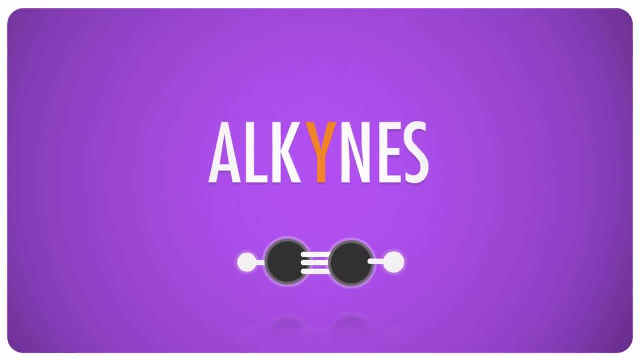 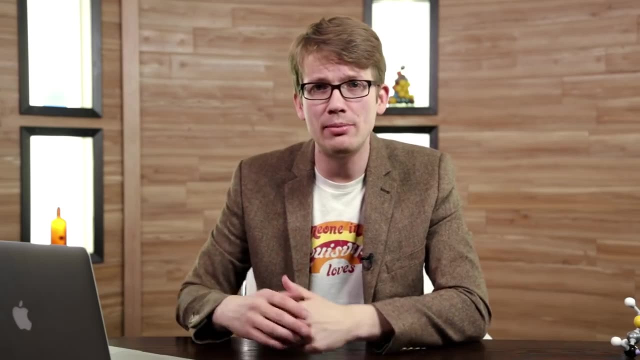 A is first, E is second and Y is third. Not too complicated, I hope. And it's actually pretty nice that the words are so similar, because it means we can reuse all of those old alkane rules. The prefixes remain the same, but the suffixes change in some fairly easy-to-predict ways. 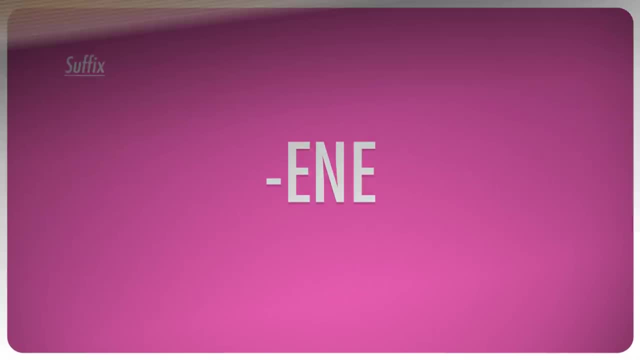 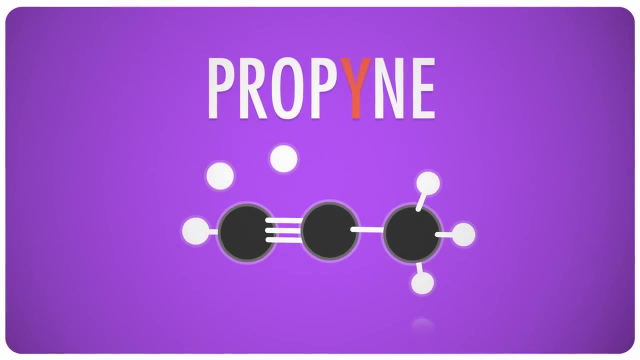 Hydrocarbons that have one or more double bonds end in "-ene", while the ones that have triple bonds use the suffix "-yne". So a compound with three carbons and one double bond would be propene. three carbons and one triple bond propyne. 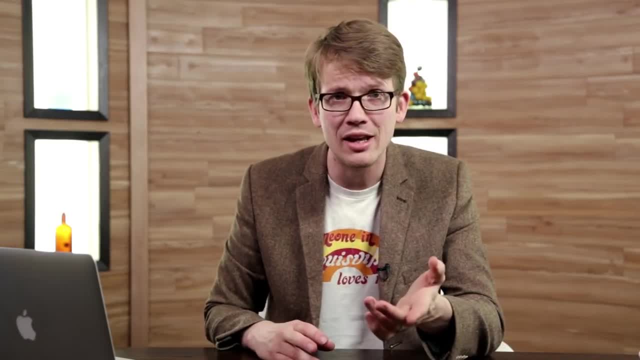 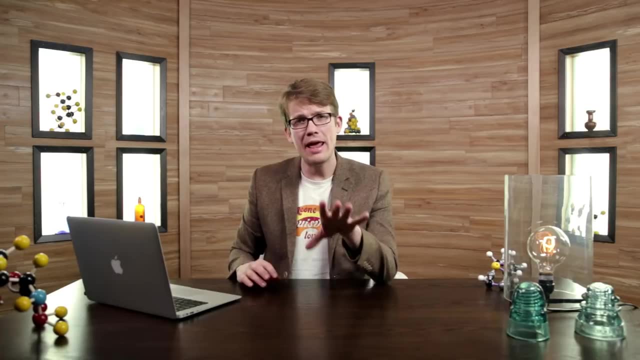 All the other naming rules apply to alkenes and alkynes too. For instance, the main carbon chain, the longest one, is numbered in such a way that the various components, including the double bond, have the lowest numbers possible. Now the bonds and alkenes have a few tricks up their sleeves, and it's not as simple as 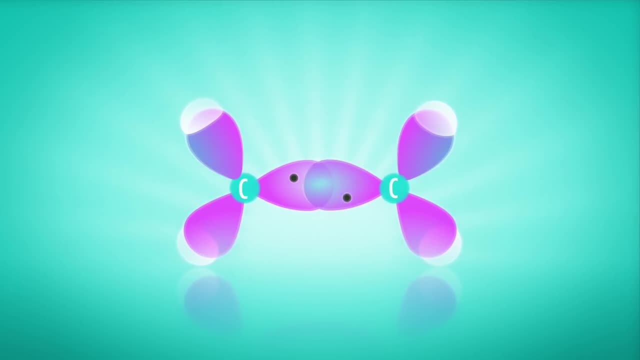 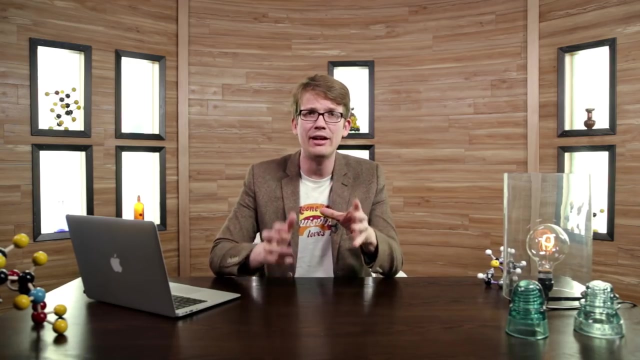 you might imagine. Single bonds, also called sigma bonds, are pretty simple and carbon atoms attached by them can rotate around the bond freely. That may not sound like a big deal at first, but alkenes and alkynes don't have that kind of freedom. And that simple fact has a huge advantage. Single bonds consist of a sigma bond and a pi bond. That pi bond bridges the sigma bond, locking it in place. so whatever's attached to the other sides of the carbon atoms can't change their orientation with respect to each other. 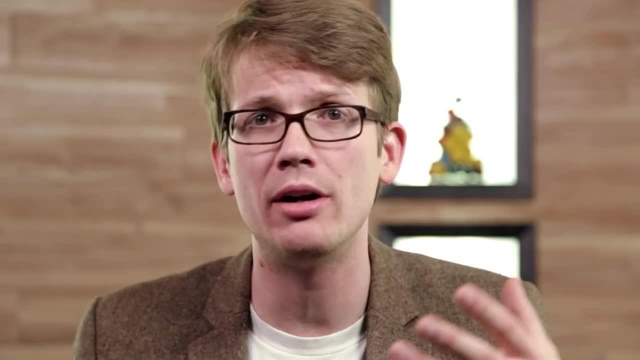 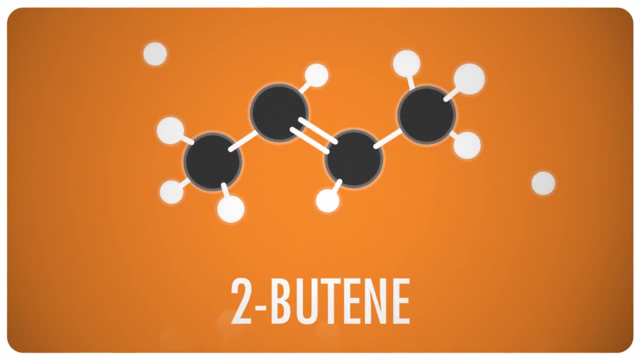 If all of the things attached to those carbons are the same, it doesn't matter. But if the parts are different, it's possible to have two totally different isomers of the same compound. Let's build an example for ourselves. Two butene should suffice, so it starts with bute. 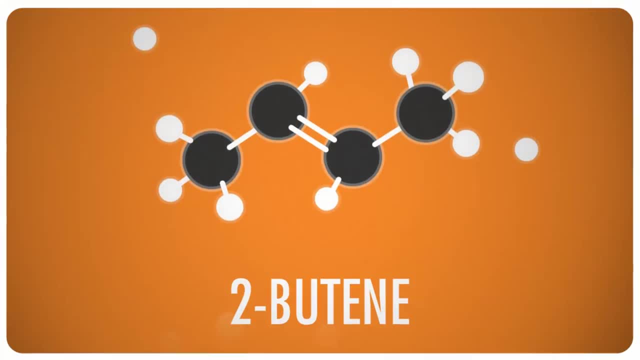 so it has to be a four-carbon chain. It ends in "-ene", so it needs to have a four-carbon chain. The two tells us that the double bond starts on the second carbon. So we've got our structure, Or do we? 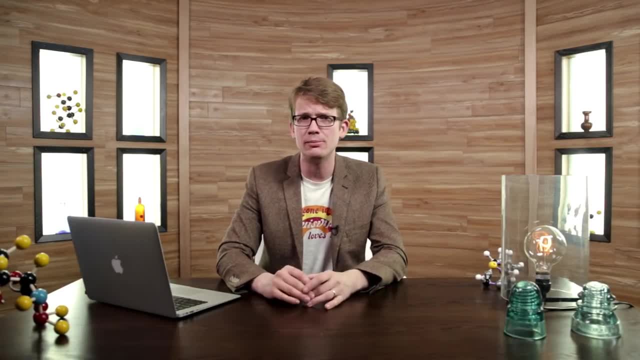 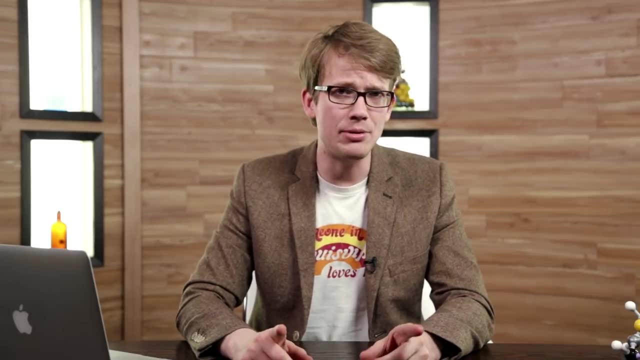 With the information we have, this two butene could be one of two different isomers: one with the methyl groups on the same side or one with the methyl groups on different sides. They're not structural isomers like n-butane and i-butane. Instead, they're what we call. 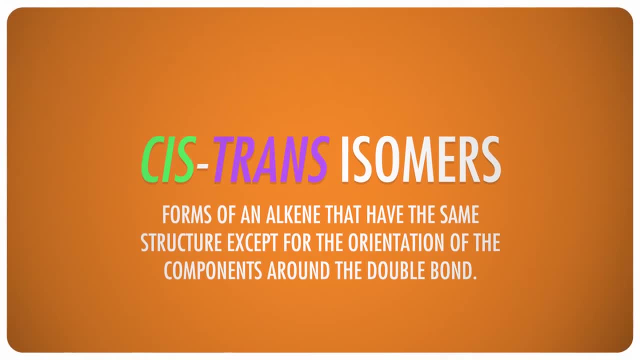 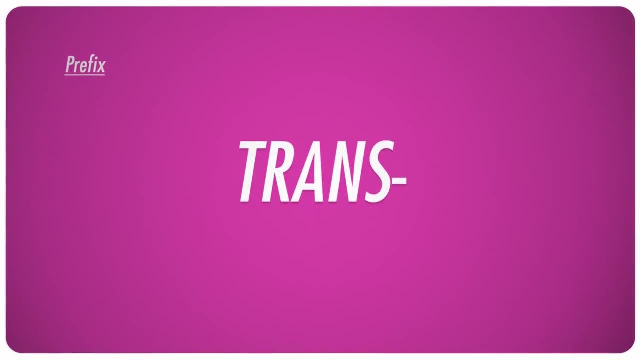 cis-trans isomers. These have the atoms in the same positions on the molecule, but the atoms are oriented differently in space. Cis comes from a Latin word that means on the same side, and trans is Latin-based prefix that means across, If the matching groups are on the same side of the double bond, like this we call it. 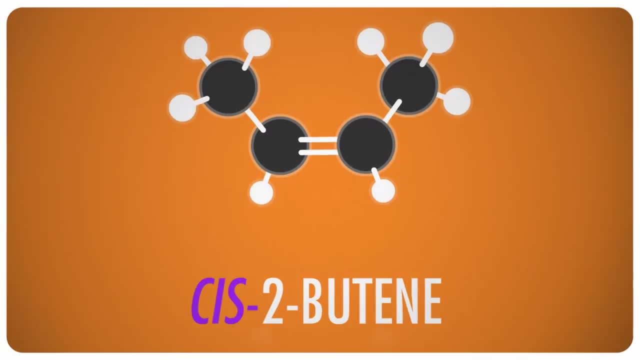 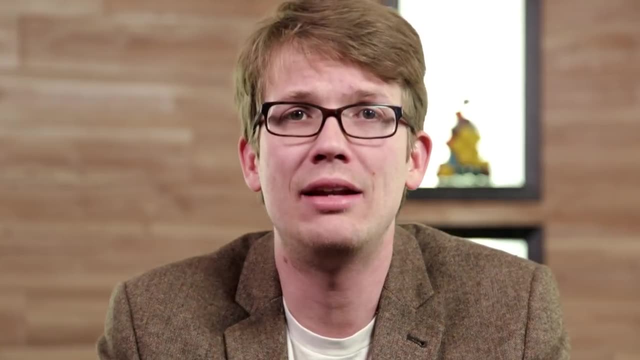 cis-tube butene, and if the two components are across from each other, it's called trans-tube butene. Note, by the way, that organic compounds cannot switch from cis to trans or the other way around. You would have to break the pi bond and thus the entire molecule to rotate. between isomers. The same rules apply no matter what's attached to the double bond. It might be a long hydrocarbon chain or a halogen or an oxygen. All that matters is whether the matching components are next to each other or across from each other. 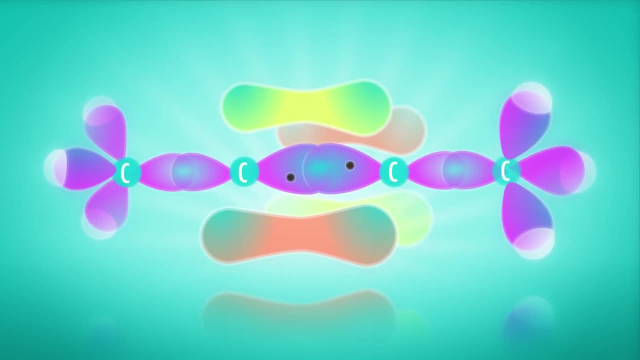 The triple bonds and alkynes, meanwhile, are composed of two different compounds, and they are composed of one sigma bond and two pi bonds for a total of three bonds. The pi bonds prevent the triple bonds from rotating here as well, but triple-bonded carbons 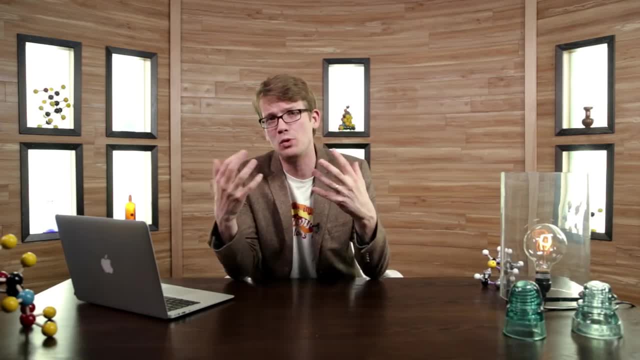 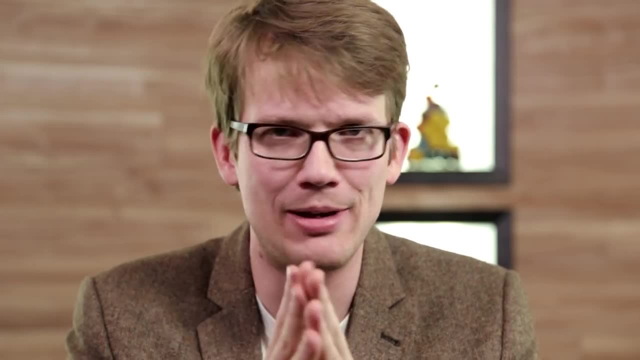 can only bond to one other atom. so even if it could rotate, nothing would change. Thus, no isomers with alkynes. Phew, Okay, I'm done describing. for the moment Let's talk about some actual chemistry. Pi bonds are significantly more unstable than sigma bonds, so double and triple bonds are 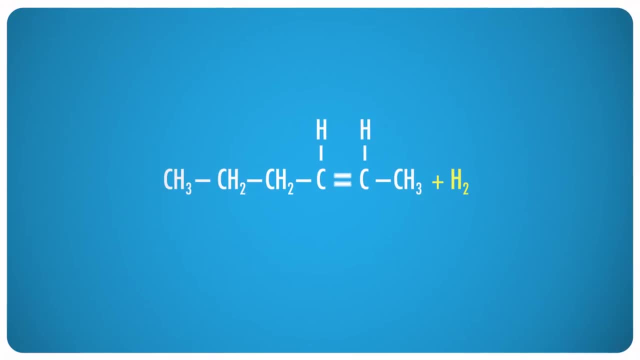 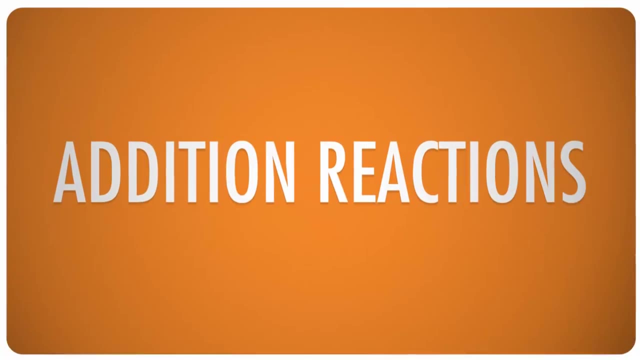 pretty easy to break, opening the doors for some good chemistry. Certain reactions open up a double or triple bond to insert various atoms. Some atoms leave only a single bond between the carbons. These are called addition reactions because atoms are added to the carbons that were previously double-bonded. 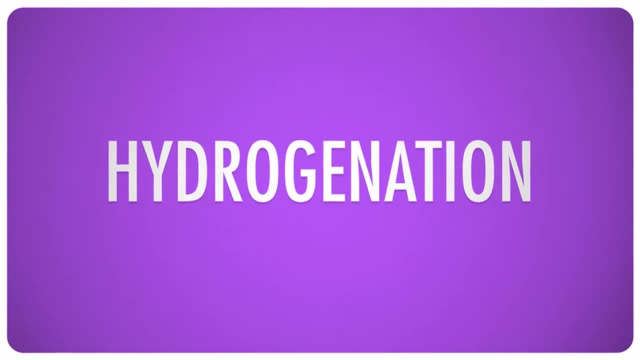 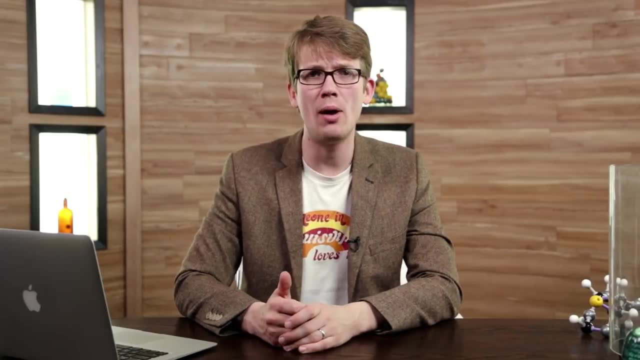 Probably the simplest addition reaction, and one that you've heard of, is hydrogenation, in which a molecule of hydrogen- H2, is added across the bond. To do this, a metal catalyst like platinum is usually required to help break the H2 apart. 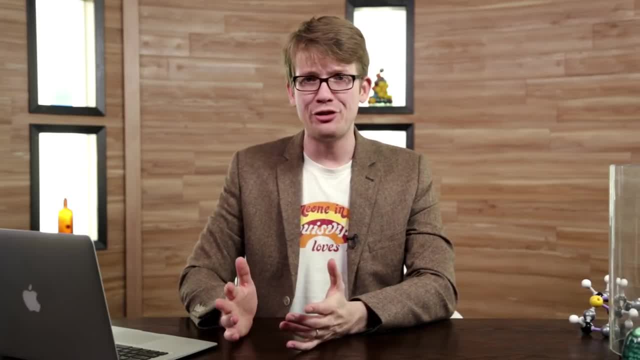 because that bond is very strong. But once that's done, the hydrogen atom is readily attached to the hydrocarbon molecule, converting a double bond to a single bond. Other molecules can break that double bond as well, If a halogen, such as bromine, is. 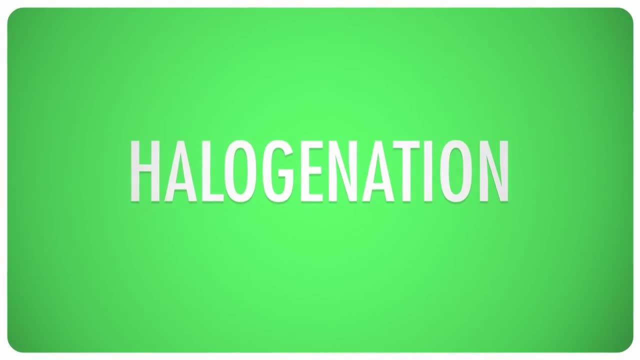 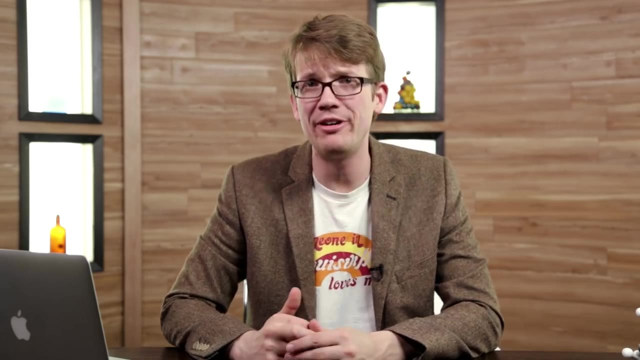 added in the place of hydrogen. the reaction is called halogenation, A water molecule hydration, oxygen gas oxygenation. You get the idea. The point is that double or triple bonds can be opened up fairly easily. Alkenes can be made into alkanes and alkynes can become either alkenes or alkanes, depending. 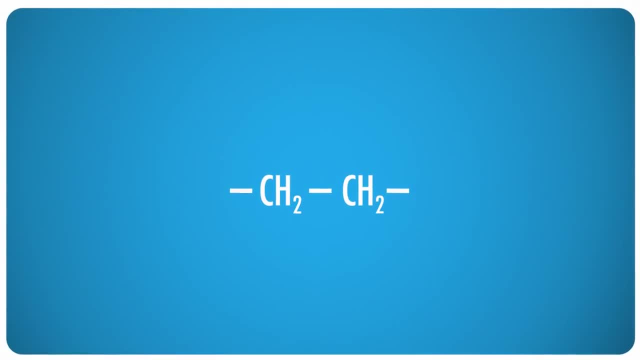 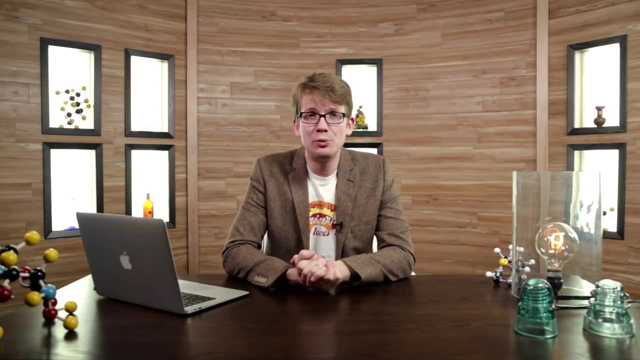 on how many atoms are added, And those opened bonds can also provide connections for carbon atoms to attach to each other too, opening the door for polymerization, which we shall talk about soon enough. Now, using all of these words we have learned today, let's apply some to our society's ubiquitous 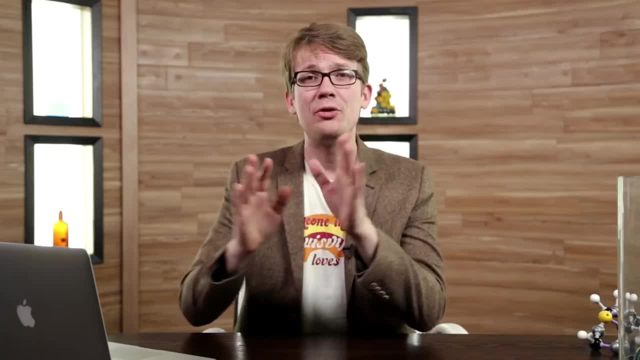 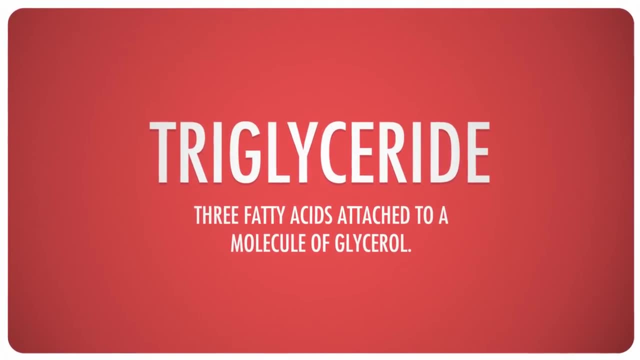 fat lingo. First, though, what is fat When three fatty acids- and we will talk about their structures more specifically in a later episode- are bonded to a molecule of glycerol, that is, a triglyceride? That's the stuff. 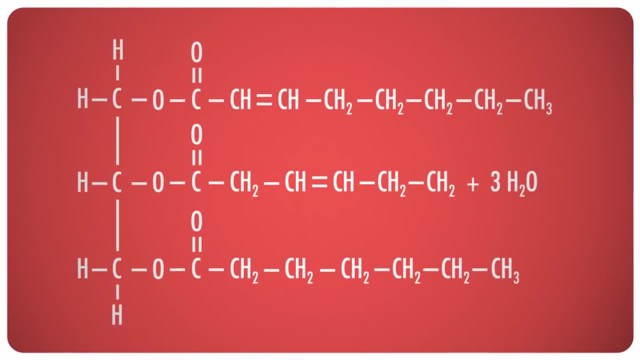 that we're generally talking about when we say fat, The fatty acid chains. they have long hydrocarbon chains are what we're mostly concerned with here. They can be alkanes or alkenes, sometimes even rarely- alkynes. 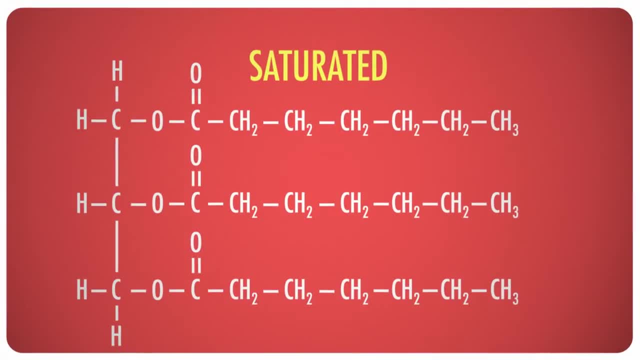 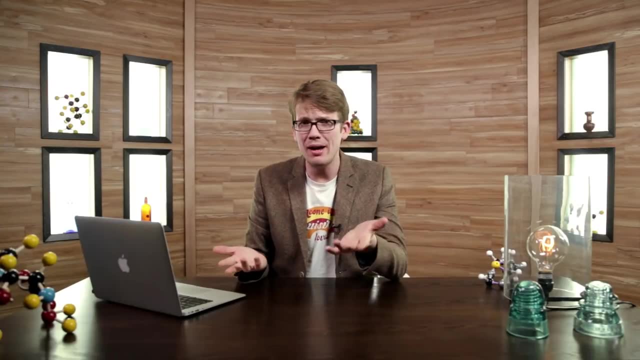 So we've heard of saturated fats. What does that mean? It means no double bonds. All of the carbon chains are alkanes and it has as many hydrogens as possible. It's saturated. That means that there are no unstable pi bonds, so they tend. 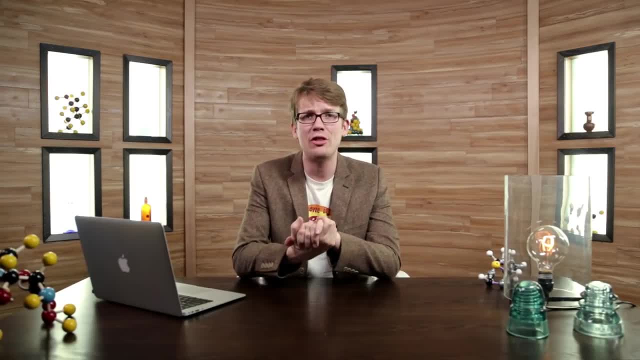 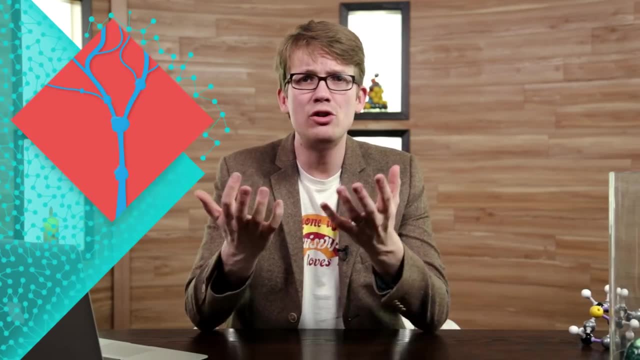 to have longer shelf lives. They're also able to lay flat against each other, making them more likely to be solid at room temperature. The bad news is that they're kind of hard for your body to do chemistry with, since they're so stable, so they often just stick around in your body clogging stuff up. 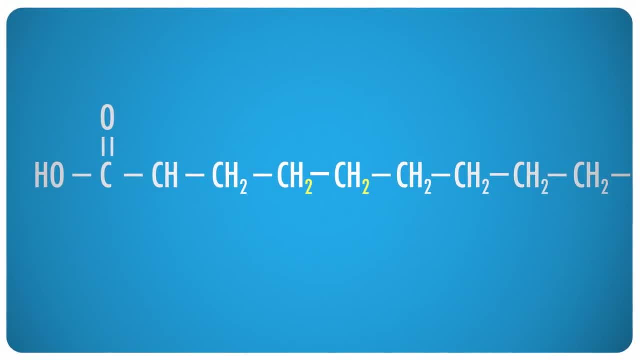 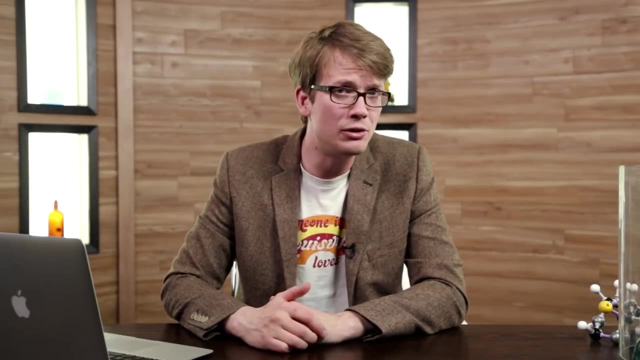 Now what about hydrogenated oils? Vegetable oils are generally polyunsaturated fats, meaning that they have lots of double bonds, or at least more than one. They're much healthier for us than saturated fats, and they're also generally cheaper, since saturated fats are. 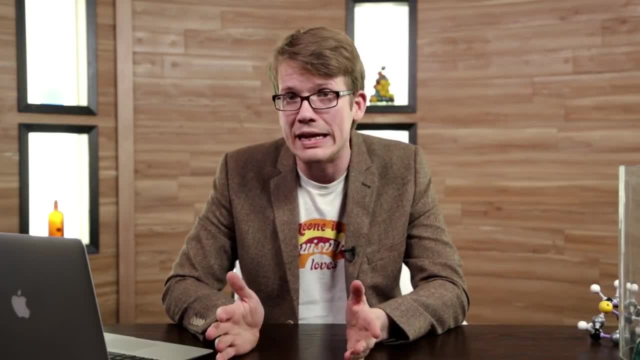 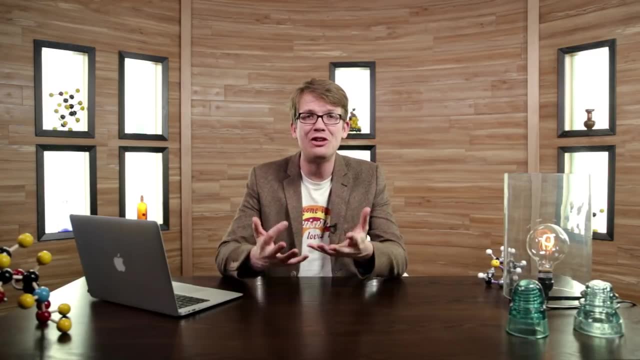 mostly made by animals, which are notoriously difficult to maintain, But they're also less stable and are usually liquid at room temperature and thus harder to spread on your toast. Food chemists use hydrogenation to saturate the unsaturated fat, making it spreadable. 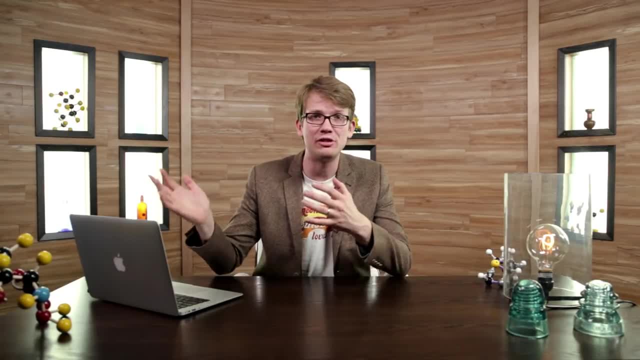 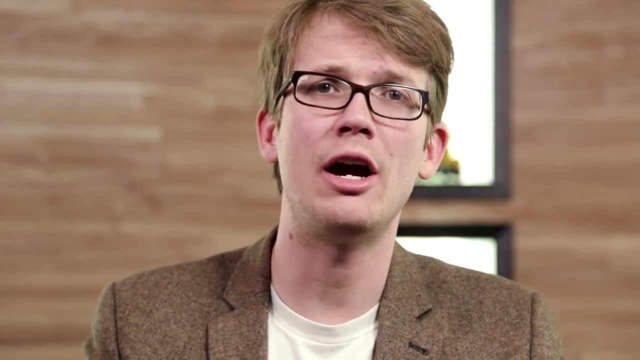 and also stabilizing it, And since it's made from vegetable oil instead of animal products, it's much cheaper to create. Sometimes the oils are fully hydrogenated, creating saturated alkanes, and sometimes they're just partially hydrogenated, usually leaving just one double bond in the fatty. 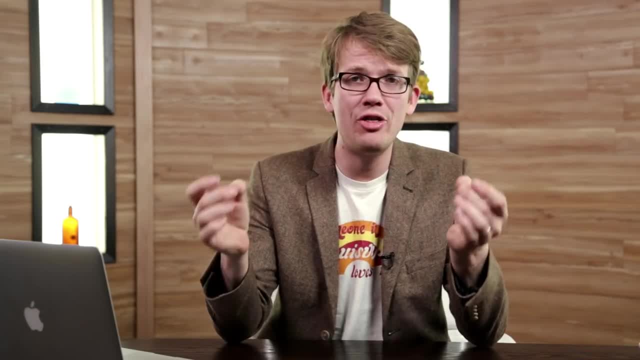 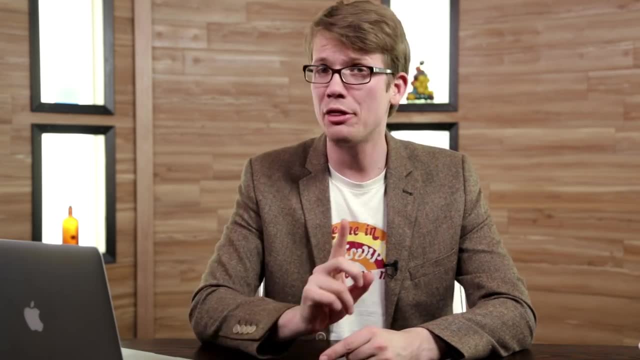 acid chain, creating a monounsaturated fat. Now, it's not just whether or not there are double bonds. The location of double bonds also has an effect on what your body can do with the molecules, which leads me to omega-3s. 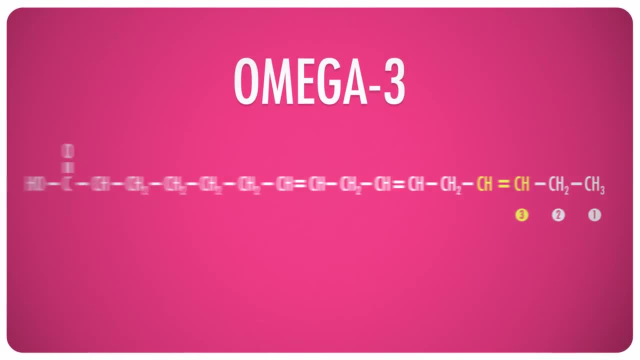 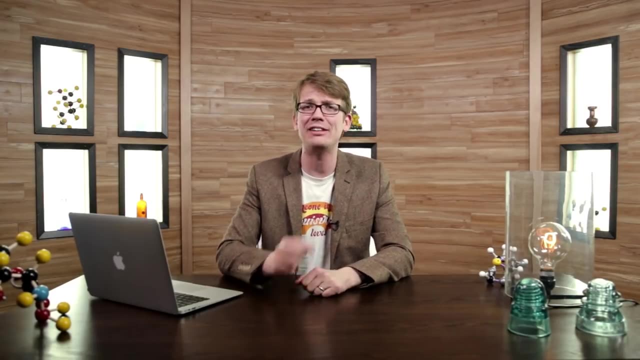 Omega-3 refers to a specific location of the double bond, three carbons from the end, or omega, of the fatty acid chain. Your body is completely incapable of making this sort of fatty acid, and yet it needs them to survive, so you have to eat them. 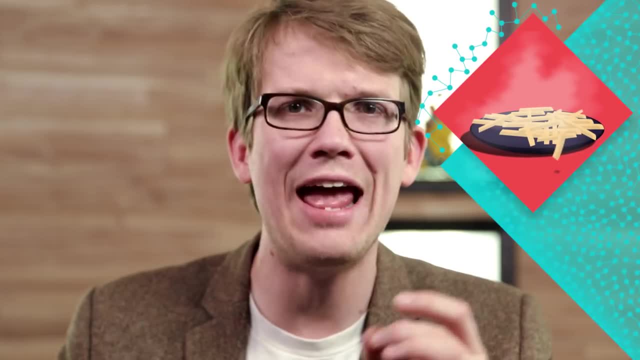 A final question: what can you tell me about the dreaded trans fats? Well, we know that they're unsaturated alkanes, but they're not the only ones that are unsaturated. They're called alkenes because saturated fats don't have double bonds and thus can't have cis. 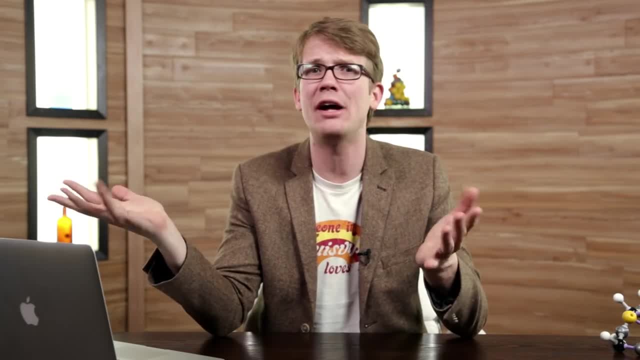 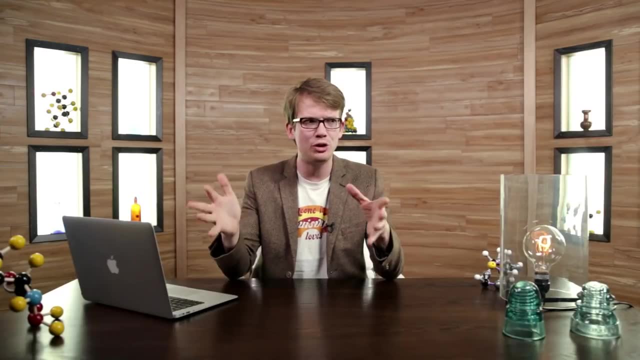 and trans isomers. But we also know from every advertisement about healthy food that probably isn't that healthy ever- that trans fats are really bad. So it's an unsaturated fat but it's really bad for you. That doesn't really jive. What's going on? 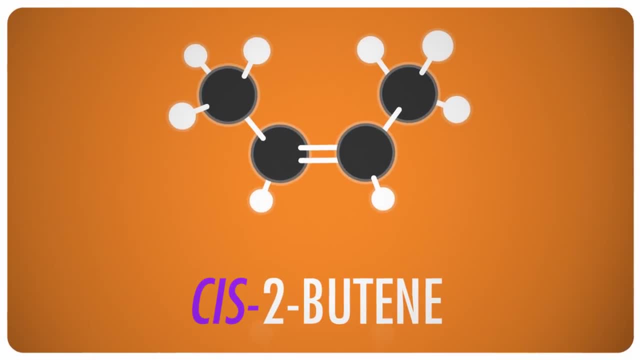 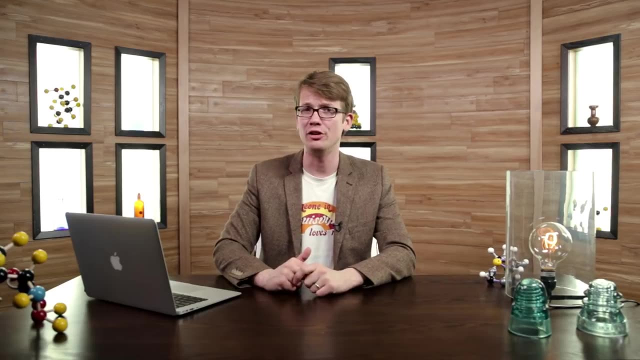 Well, almost all natural unsaturated fats are cis fats, which our bodies are prepared for and know what to do with. Trans fats are created by partially hydrogenating vegetable oil on a cheap path to tasty fat without all that unsightly saturated fat on the diet.